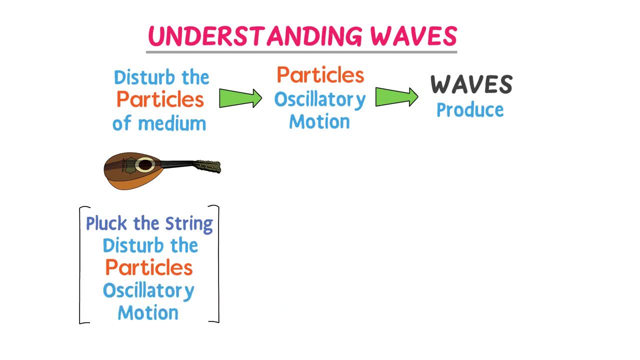 start oscillating about their mean position and sound waves are produced. Secondly, heading a cup constantly. During heading, you disturb and set the particles of the string in the medium to oscillate about their mean position. As a result, sound waves are produced. 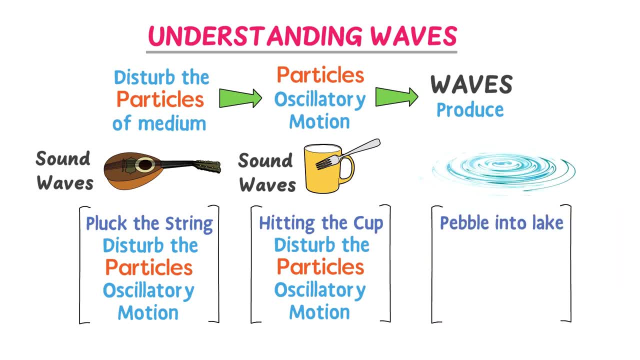 Thirdly, when you throw a pebble into the lake, you disturb the particles of the water. They start oscillatory motion about their mean position. As a result, you observe waves across the lake. Thus, from these examples we learn that if we disturb the particles of any medium, 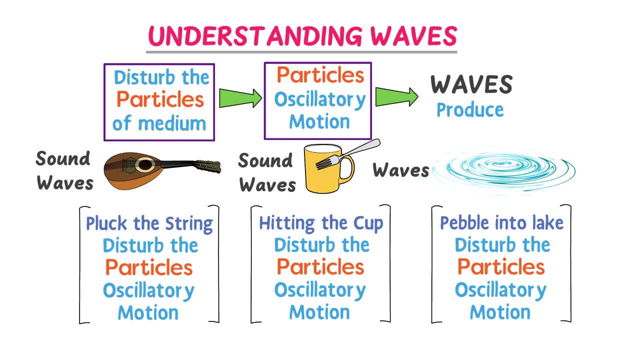 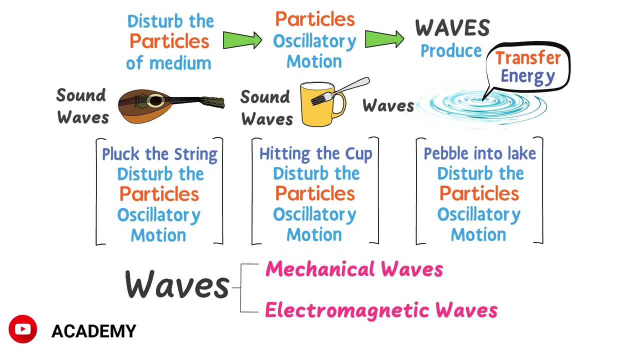 such that they oscillate about their mean position. waves are produced in the medium. Also, remember that waves transfer energy from one place to other place without transferring the particles of the medium. Now there are two types of waves: mechanical waves and electromagnetic waves. 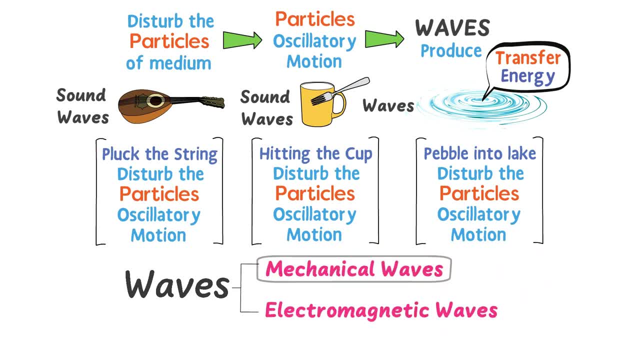 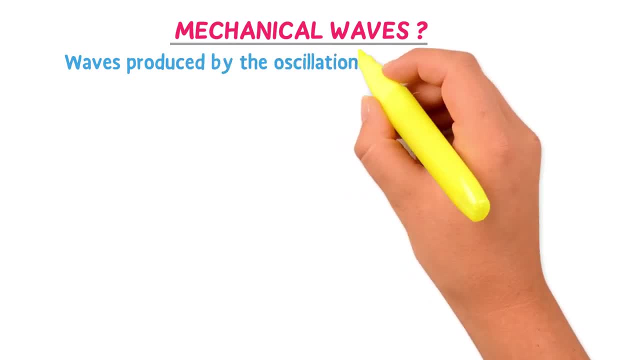 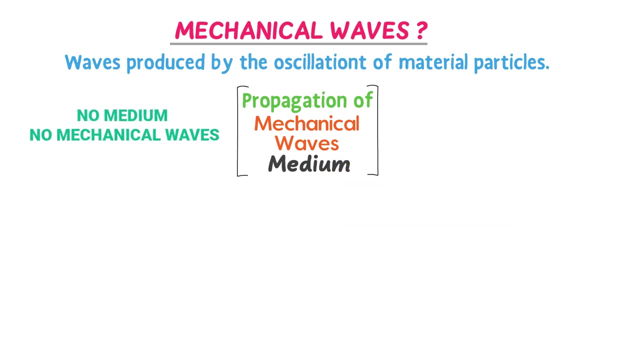 In this video, I will teach you only about mechanical waves. Now, what are mechanical waves? Well, waves produced by the oscillation of material particles are called mechanical waves. Remember that the propagation of mechanical waves requires medium. No medium means no mechanical waves. 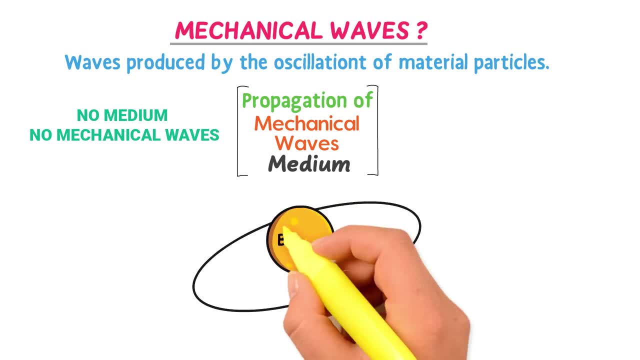 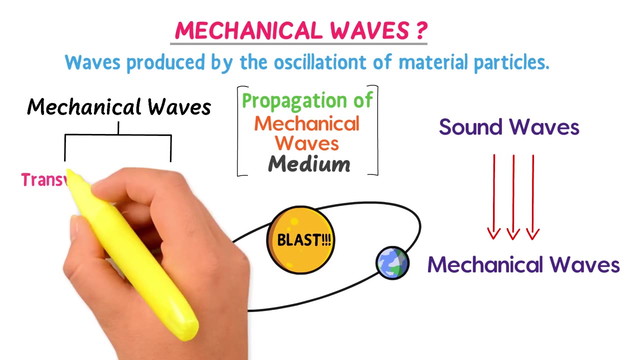 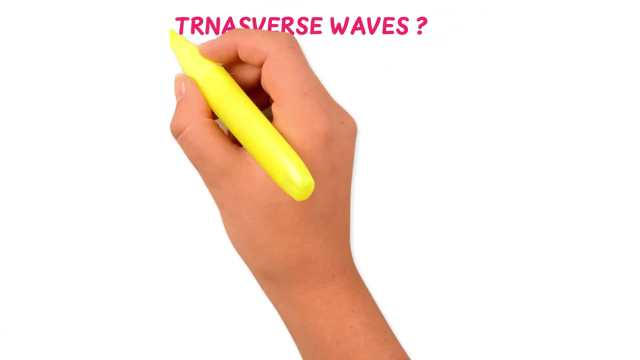 For example, we cannot receive the sound of the sound of mechanical waves Explosion outer in the space. It is because sound waves travel in the form of mechanical waves. Mechanical waves are further divided into two types, like transverse waves and longitudinal waves. Now let me teach you about transverse waves. 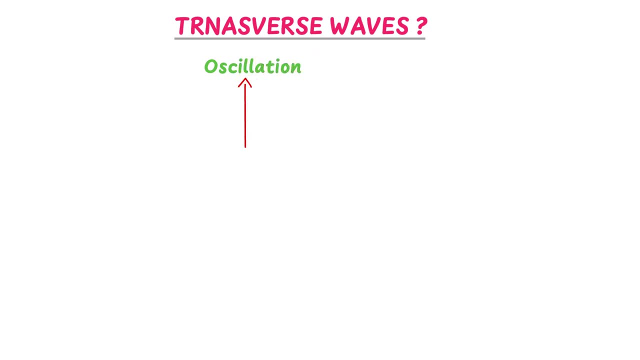 If the oscillations of particles are in y direction and motion of the wave is in x direction, we call it transverse wave. Let me repeat it: If the oscillations of particles are in y direction and motion of the wave is in x direction, 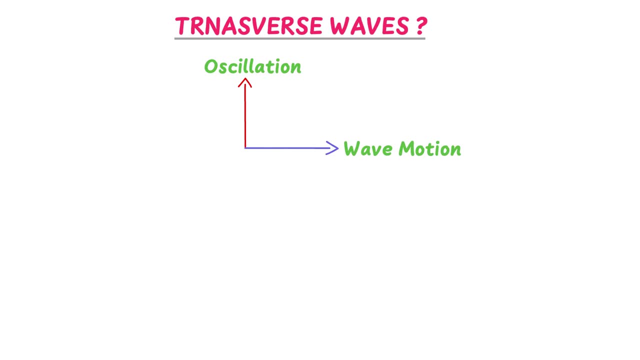 we call it transverse wave. Note it down that in transverse waves the angle between oscillations of particles and wave motion is 90 degree. They both are perpendicular to each other. For example, consider the waves produced in this lanky spring. 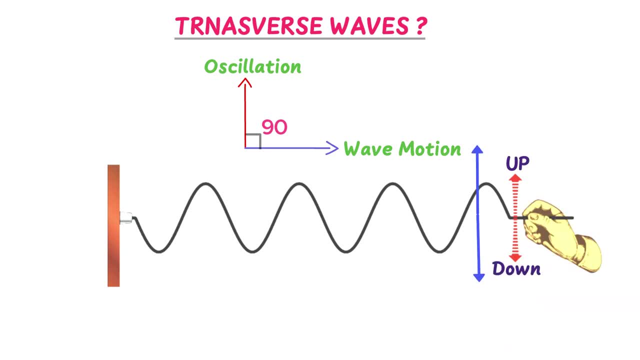 Your hand moves up and down in y direction, while the wave move in x direction. So it is an example of transverse waves. Transverse waves are made out of consecutive crests and troughs, The part of wave above mean or equilibrium position. 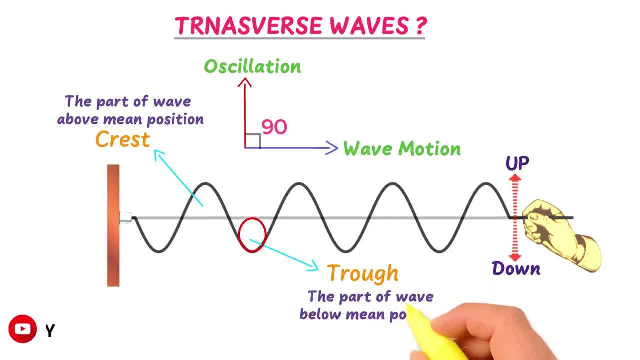 is called crust, While the part of wave below mean is called trough. below the mean, our equilibrium position is called trough. The example of transverse waves are water waves and electromagnetic waves are EM waves like X-rays, radio waves, light waves etc. 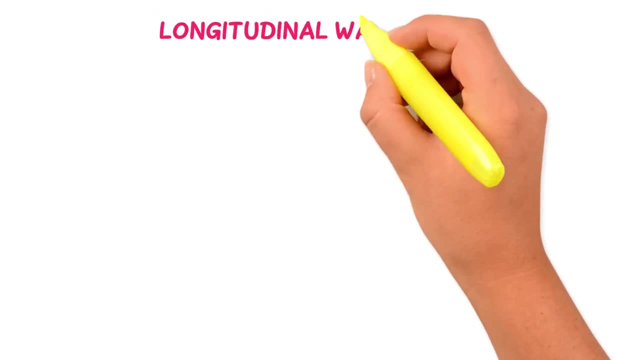 Finally, let me teach you about longitudinal waves. If the oscillations of particles are in X direction as well as the motion of wave, we call it longitudinal wave. Let me repeat it: If the oscillations of particles are in X direction as well as the motion of wave, 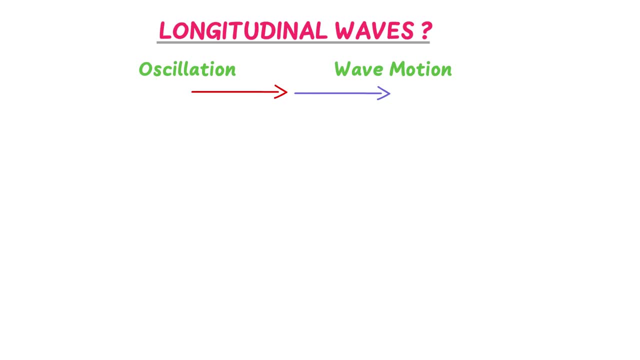 we call it longitudinal wave. Note down that in longitudinal waves the angle between oscillations of particles and wave motions, The motion, is zero degree, as they both are parallel to each other. For example, consider the waves produced in this spring. Here your hand moves back and forth in X direction, while the wave also moves in the X direction. 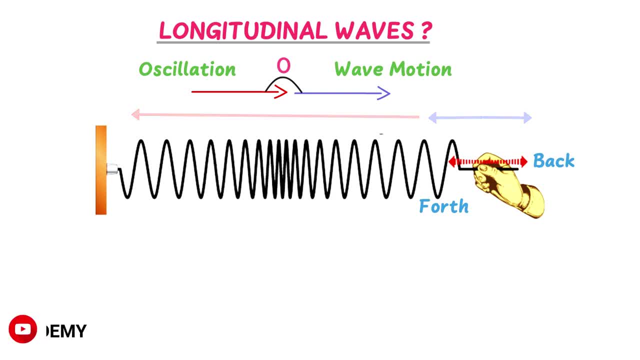 So it is an example of longitudinal waves. Longitudinal waves are made out of consecutive compression and rarefaction. The region of relatively high density and pressure is called compression, while the region of relatively low density and pressure is called rarefaction. The example of longitudinal waves are sound waves. 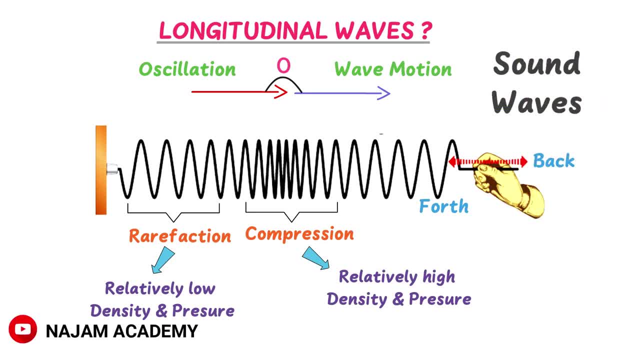 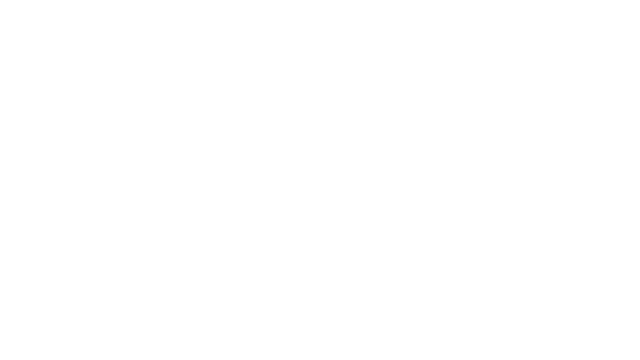 The sound we produce or hear travels in the form of longitudinal waves. Lastly, as a bonus tip, Y wave motion is also called simple harmonic wave. Well, consider the motion of transverse waves and longitudinal waves. In transverse waves, your hand or particles of the medium move up and down about their mean position.